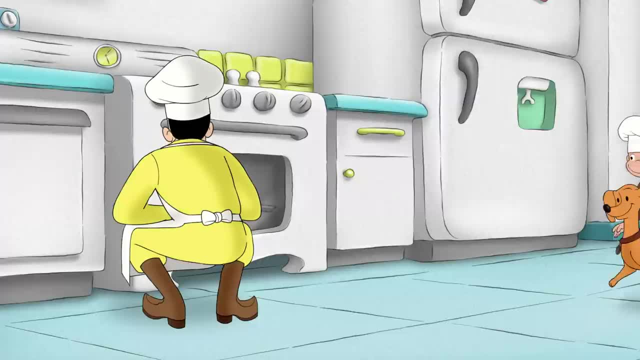 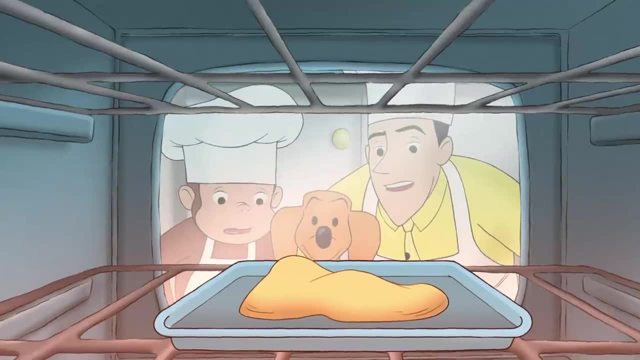 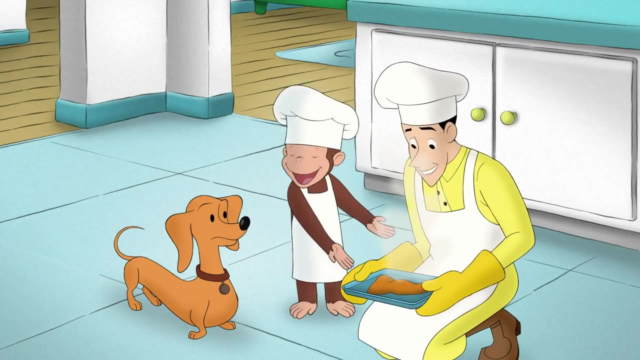 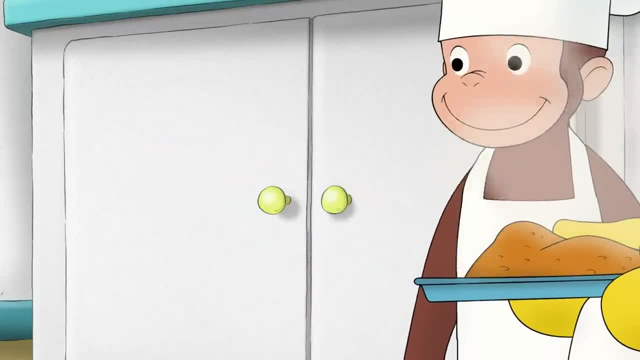 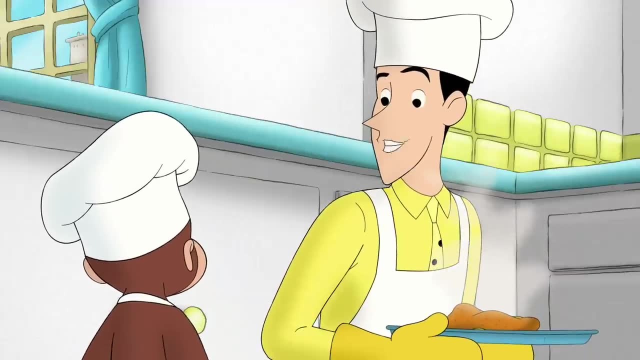 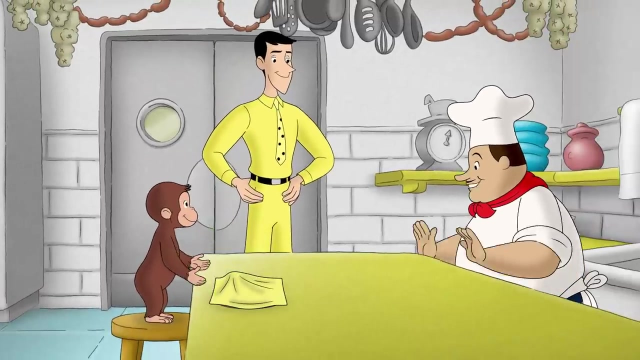 sure didn't look like it. Oh, Oh, Oh, Oh, Ah. Good idea, We should bring it to Chef to have the first taste. Woo Oh, Hey. what do you got there, Giorgio? Oh, oh. 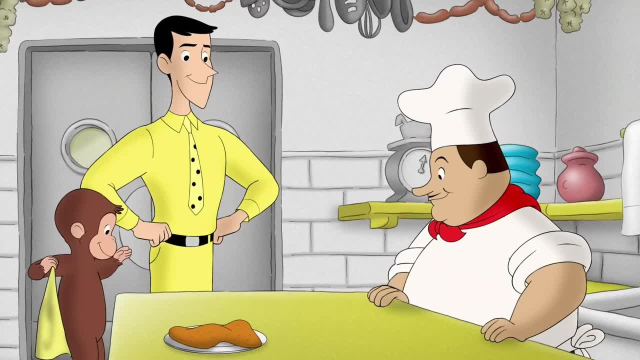 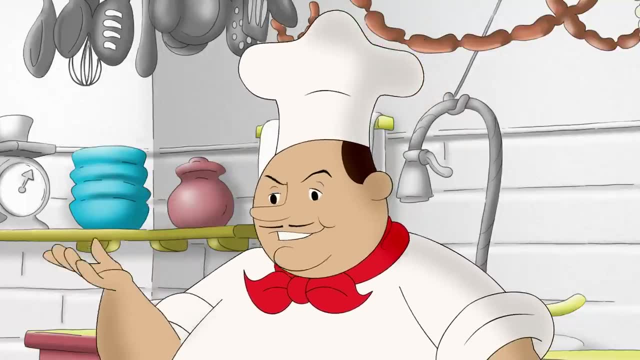 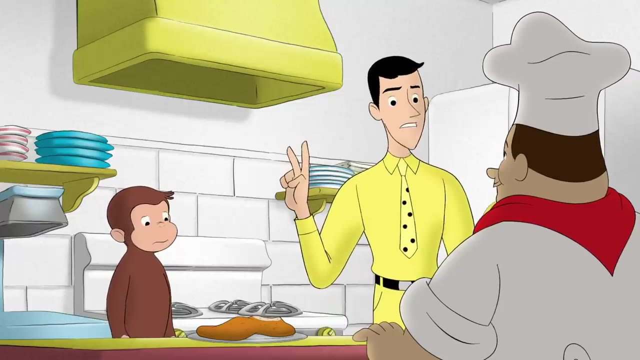 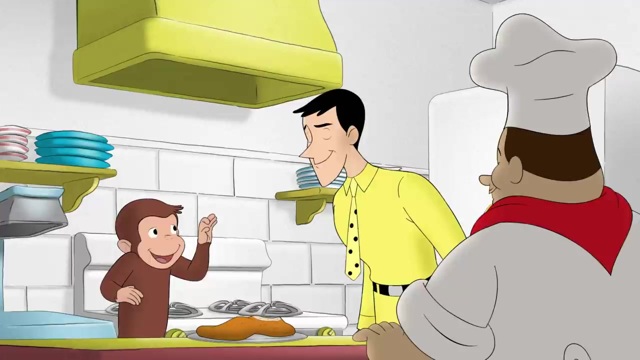 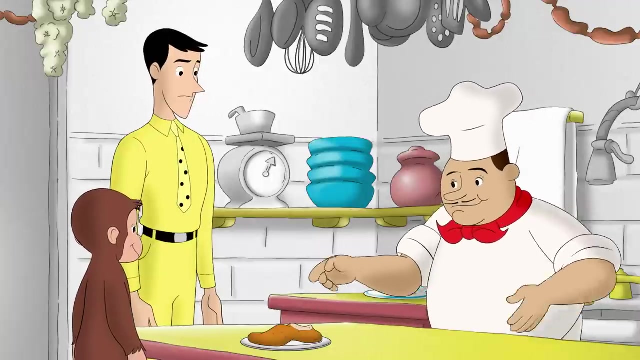 We made bread. Ah, Oh, it's very sweet. How much sugar did you use? Two tablespoons, like you said. Did you add extra sugar, George? No extra sugar. You see, Georgie, too much is going to keep the bread from rising. 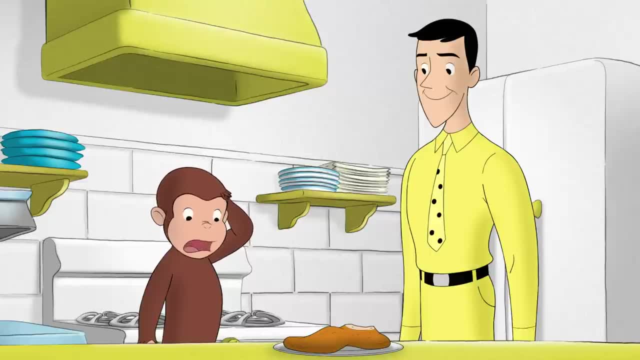 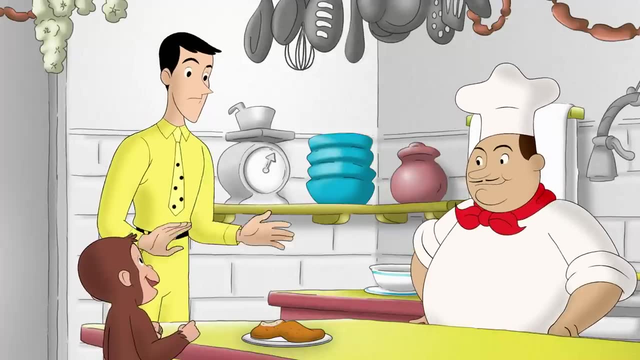 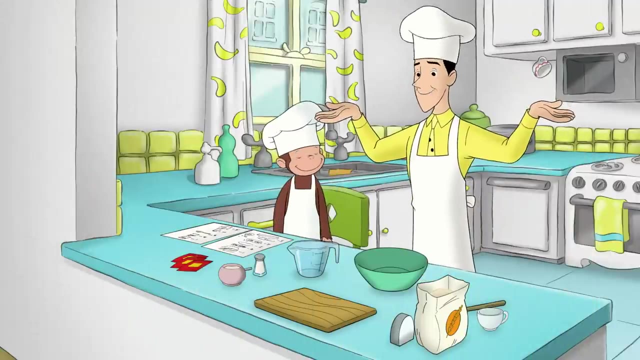 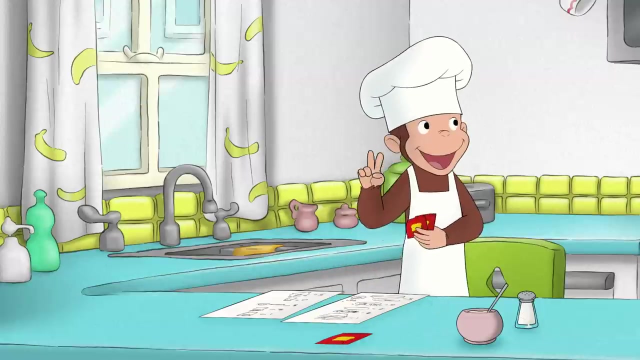 It took me a while to get it right too. You just keep trying, We will, Chef, Now let's make some great bread. Ingredient number one: water. Oh, good idea, If one packet of yeast didn't make the dough rise. 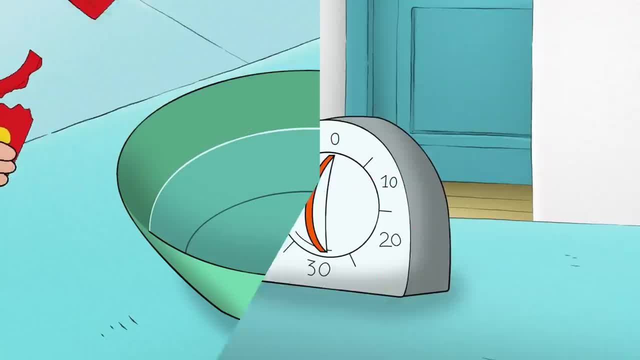 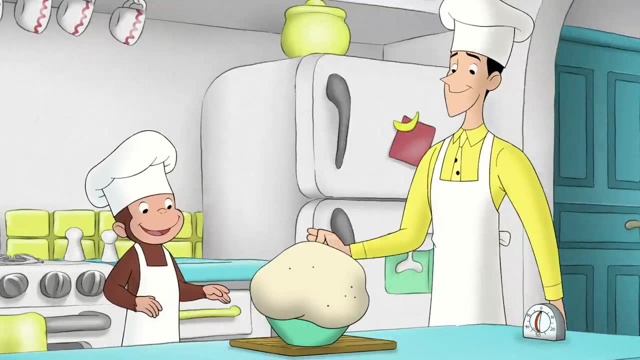 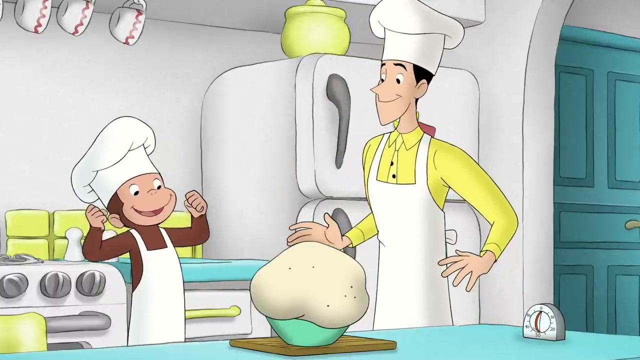 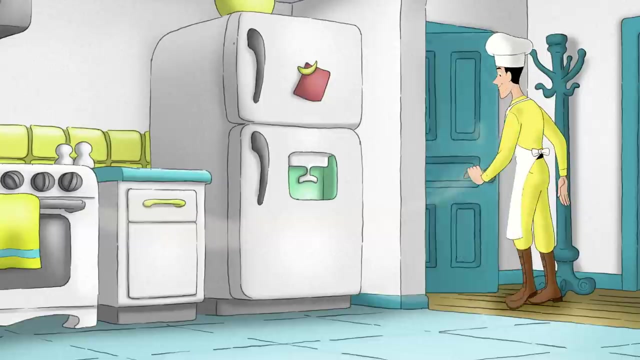 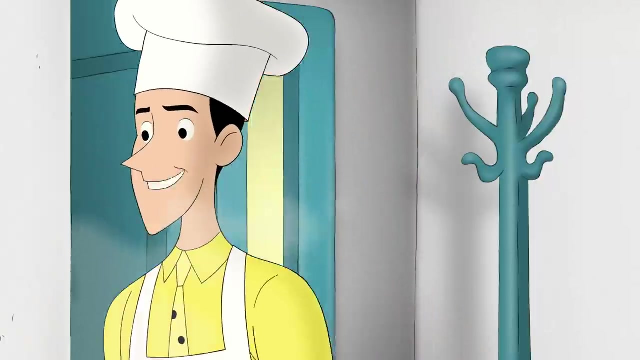 two will. Okay, let's see if it's risen. Wow, that yeast really worked. huh, Maybe we better punch it down Now we bake it. Quite a nose, you've got Hunley. It does smell good. It'll be the fluffiest bread ever. 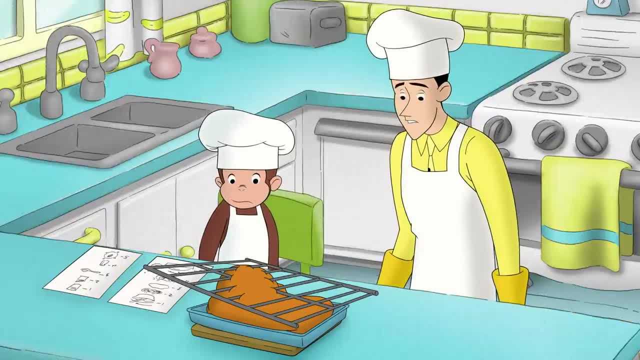 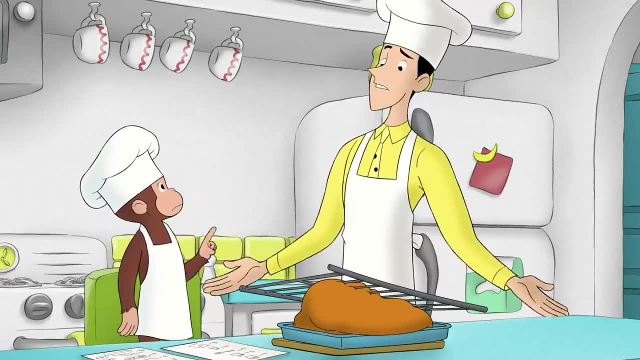 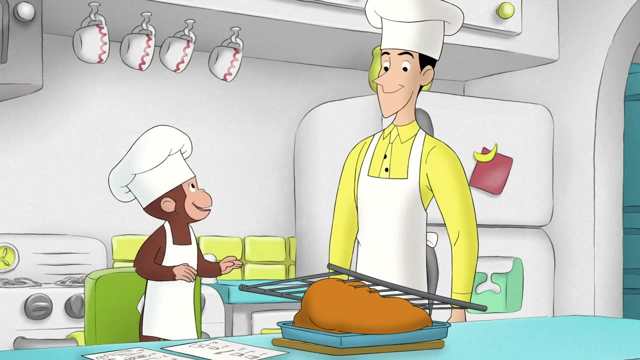 Two packets of yeast was too much. George Chef said it took a few tries for him to get his bread right. Okay, one more try, but this time let's follow Chef's directions exactly. Five, four, three, two, one.